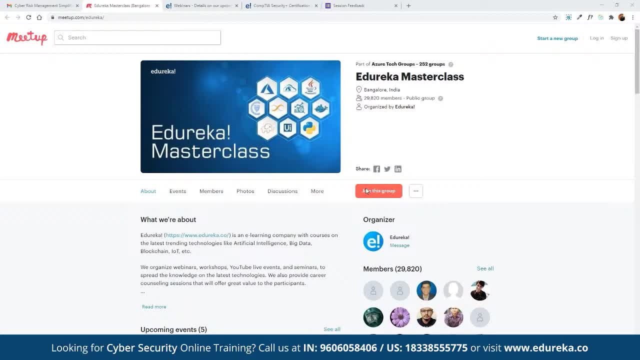 multiple webinars and live events on different topics, including blockchain, IOT, machine learning on big data and on multiple front-end and black-end development technologies. and the best part about these webinars are they are absolutely free of cost, So there are no charges involved here, And these are a really good platform for anyone who is looking to get into a specific industry vertical by learning the technology that they are interested in and that is acquired. 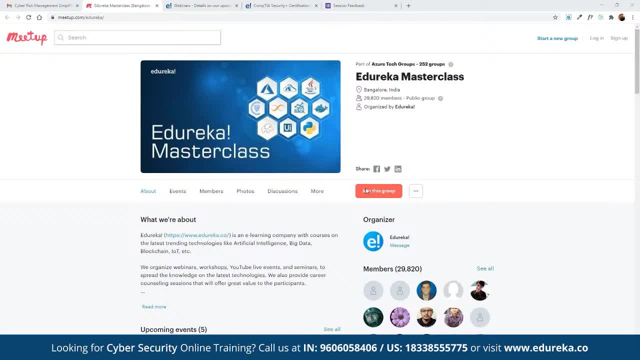 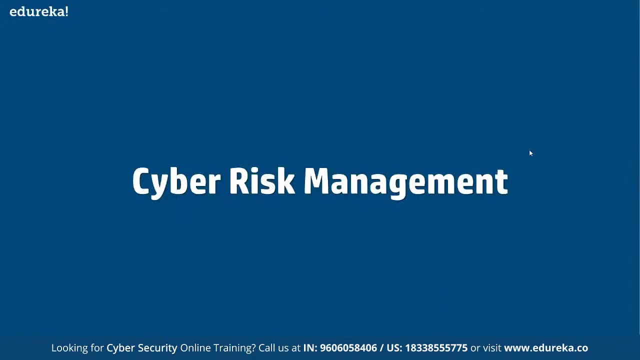 So to be a part of this community and to get the access to all the recordings as well for the webinars of the evidence that they are going to attend. So you simply have to click on join this webinar and then you will join this group and then you will be notified with the entire schedule that has been planned for the month. So let's get started. So we have gathered for our discussion on cyber risk management and to understand what exactly it is. So here we are going to discuss on the cyber risk management, What exactly it is. 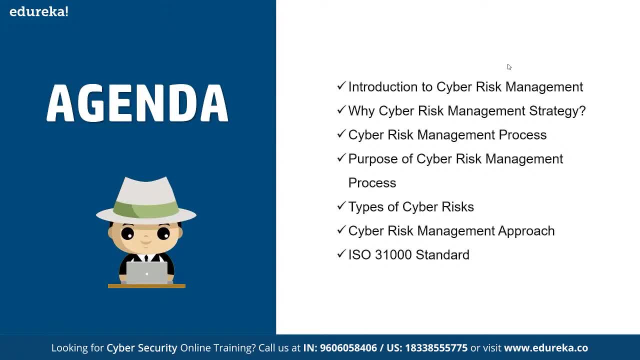 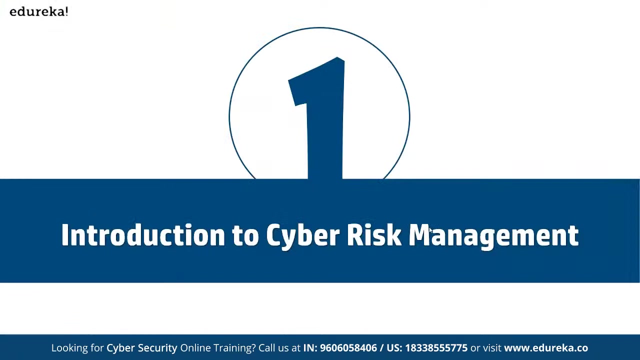 And what are the strategies involved in cyber risk management And then we are going to do to discuss on the purpose of cyber risk management. Then we are going to talk about the cyber risk, the cyber risk management approach, the ISO 31,000 standard as well. So, first of all, if you talk about the cyber risk management itself, then risk management basically is a process of identifying potential. 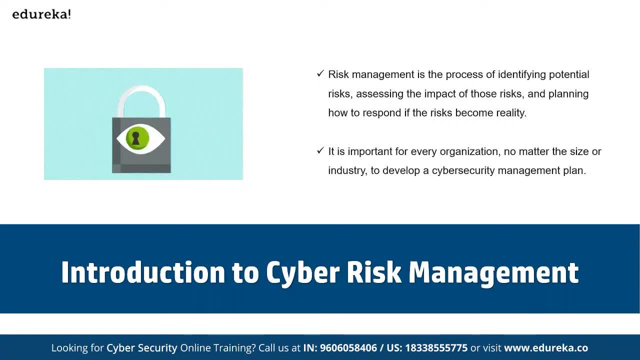 risk, assessing the impact of those risk and planning how to respond to the risk if it becomes reality. So it is important for every organization, no matter the size or the industry, to develop a cyber security management plan here. So basically, it's a concept that has been around as long as companies had assets to protect. the simplest example maybe insurance: life, health, auto and other insurance again. 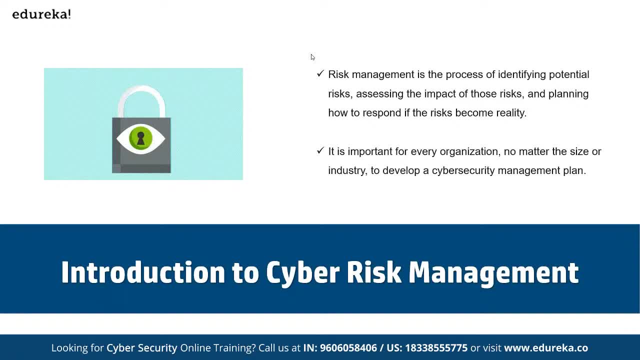 they all are designed to help a person protect against losses, right? So same way risk management also extends to physical devices such as doors and even locks to protect homes and auto and autos values, or we can say walls to protect money and precious jewels, and police, fire and security to protect against any other physical risk involved. Now, if you talk about cyber security risk management and what exactly it is, 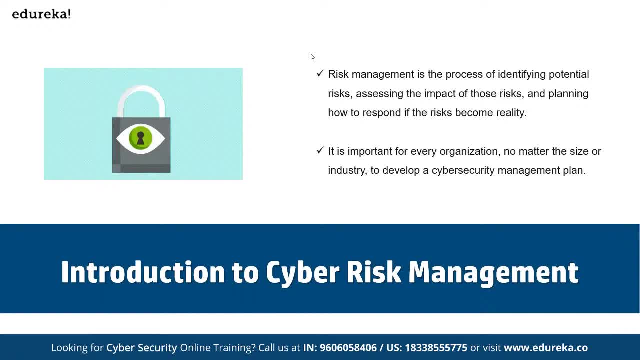 So, rather than doors, locks and vaults, IT departments rely on a combination of strategies, technologies and user education to protect an enterprise against cyber security attacks that can compromise systems, that can steal data and other valuable company information And damage and enterprises are debate reputation. So, as the volume and severity of cyber attacks grow, the need 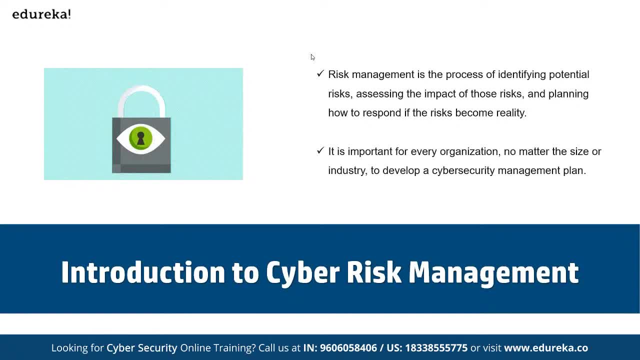 for cyber security risk management grows with it. So we can say that cyber security risk management takes the idea of real-world risk management and then it applies it to the cyber world and it involves simply identify the risk and vulnerabilities and applying the administrative actions, actions and comprehensive solutions to make sure our organization. 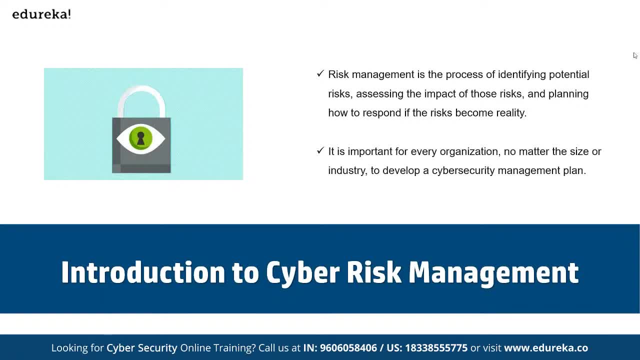 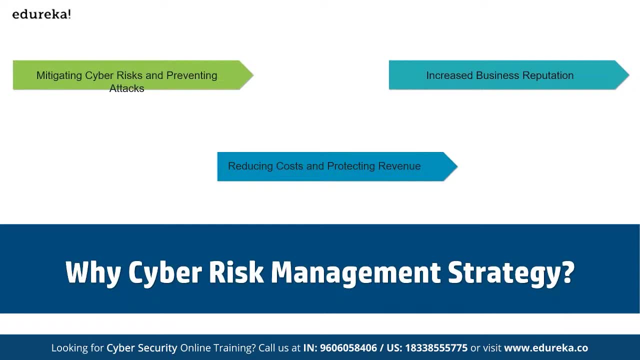 is adequately protected as well. So if you talk about us by cyber risk management, as we discussed, it simply helps us in mitigating the cyber risk and preventing attacks and it increases the business reputation, because we know we had seen that they have been multiple hacks. 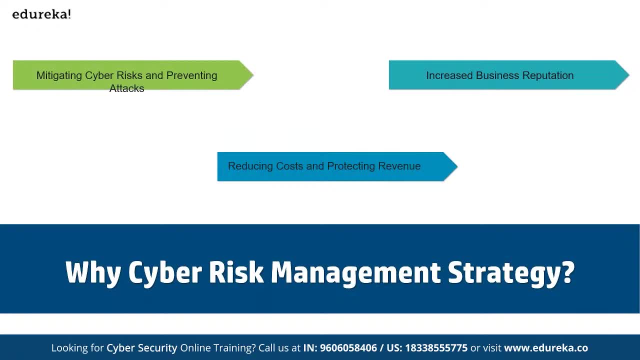 all around the domain, multiple data leaks, which has damaged the company's reputation and have caused them millions of dollars as well, And we don't want that to happen for our own company, Correct. So that is something that we can avoid and it also helps us. 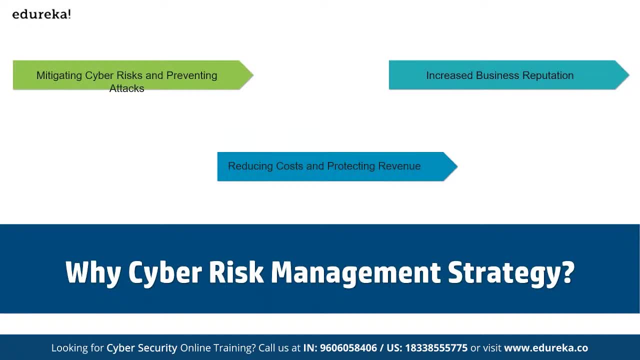 in reducing costs and protecting the revenue as well. So obviously, when we are spending on security, then we are simply avoiding the extra money that we have to pay in case our data is hacked or we experience any kind of data loss. So that is going to cost us more than spending. 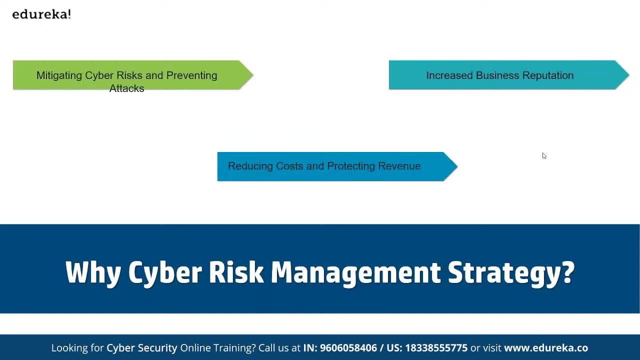 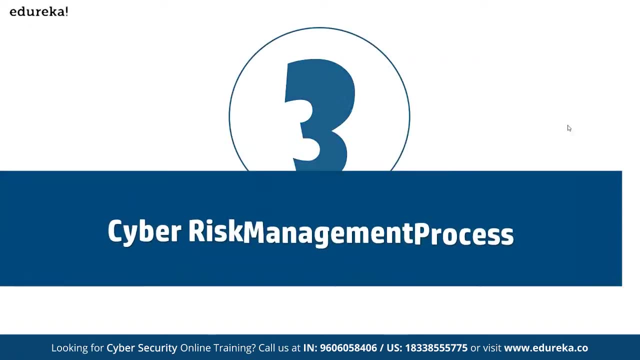 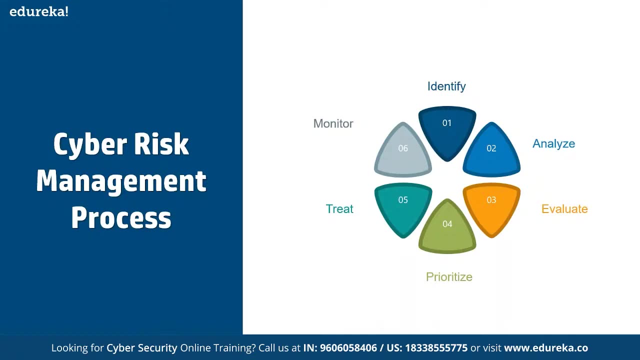 in securing these different assets, And that exactly is what cyber risk management gives to us. So if you talk about the entire process of cyber risk management, then it involves six stages here. So here we have identify, analyze, evaluate, prioritize, and then we have to treat it as well. 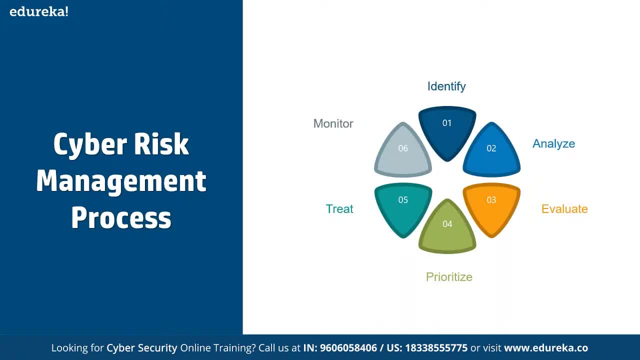 So, first of all, if you talk about the risk management process now, with starting with the cyber security framework developed from each area of the business to determine what the exact risk portion of the business should be, So if you talk about the initial steps, then the guidance software recommends using new techniques. 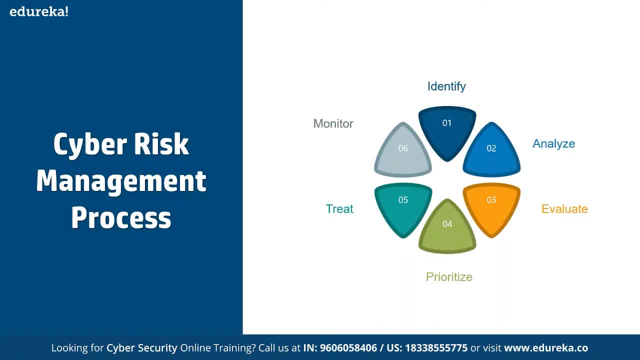 and technologies that can find and map data across the enterprise. So once the data is mapped, the organization makes better decisions on how the data is governed and reduce their risk footprint, For example. let's say, even with training and strong security culture, sensitive information can leave an organization simply by accident. 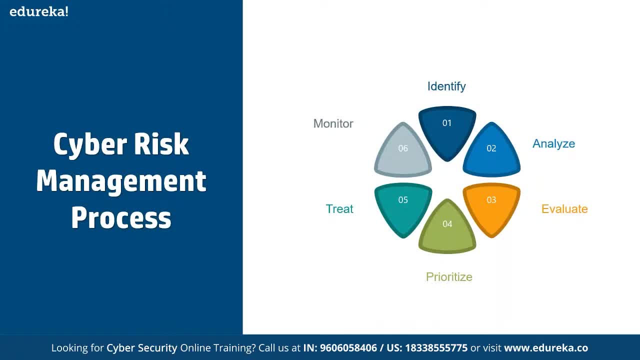 and such as data stored in hidden rules in spreadsheets or included in notes with the employees, presentations or long email threads as well. So scanning the enterprise for sensitive data at rest and then removing any data stored where it does not belong greatly reduces the risk of accidental loss of sensitive data. 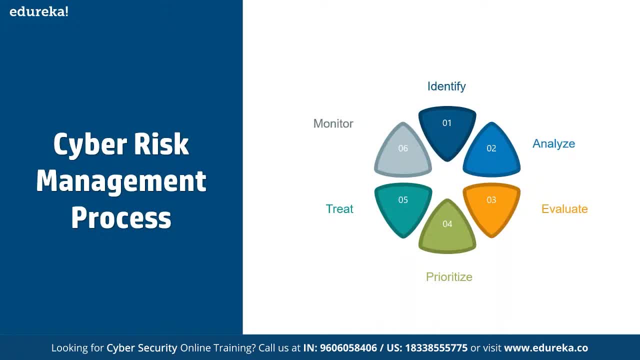 because accidents they do happen, right. So, even though we have the expert team again, still we are human, So we are bound to make multiple mistakes. So the company, that's just Deloitte now. it simply recommends that the risk management process. 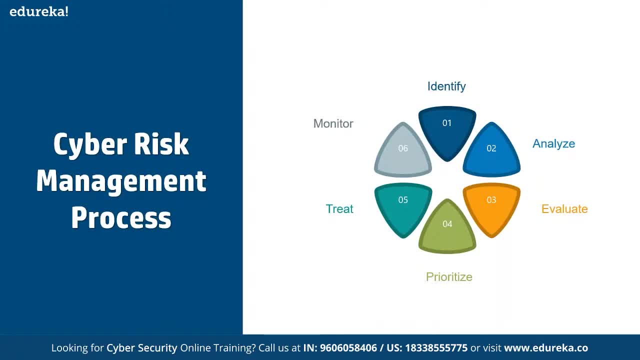 something called as a capability maturity model approach as well, where we have multiple levels as well. Like we have the initial level, We have repeatable, defined, manage and optimizing. So, first of all, if you talk about the entire process here, then in terms of identifying- so we have to identify the risk. 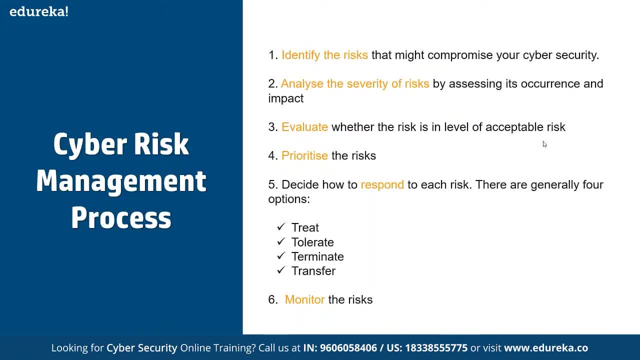 that might compromise our cyber security. For example, if you talk about any application infrastructure, then we have the app. Navi may have multiple Vulnerability is in the application structure against application code. We may have multiple vulnerabilities in the network. We may have multiple vulnerabilities. 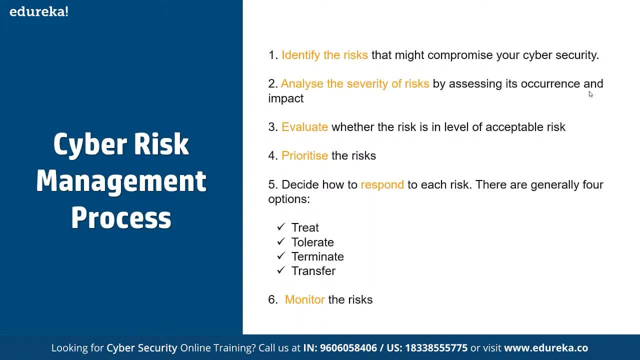 in the infrastructure, in the third-party gate, We can say the API that we are using. so they are multiple threats involved, multiple vulnerabilities involved, and we have to ensure that we are removing those kind of vulnerabilities when we are working on the, on the plot, on the process of identifying risk. and then we have 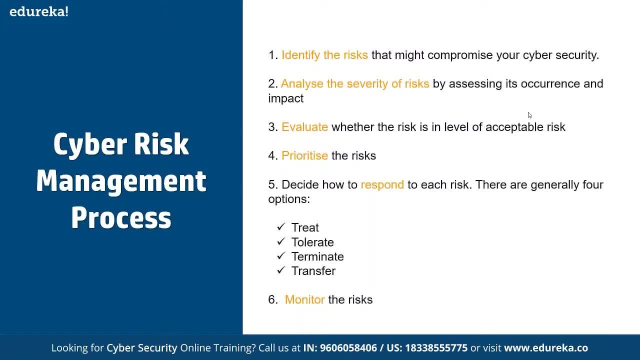 to analyze the severity of the risk as well by acts, by assessing the its occurrences and the impact as well, And then we have to evaluate whether the risk is in the level of acceptable risk. We have to prioritize the risk as well. That means which one needs to be solved. 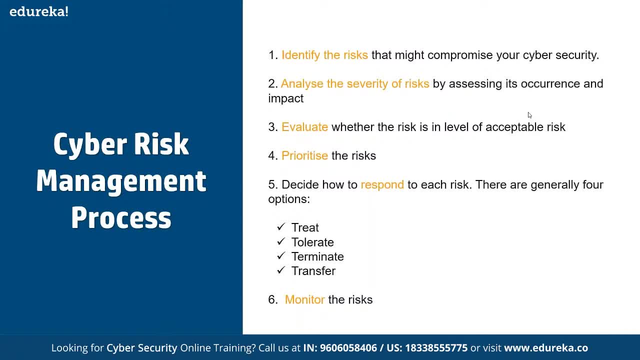 or which one needs to be addressed first and which one can be kept for later. And then we have to decide how to respond to each risk. They are generally four options: We have to treat, tolerate, terminate and transfer, and then we have to monitor the risk as well. 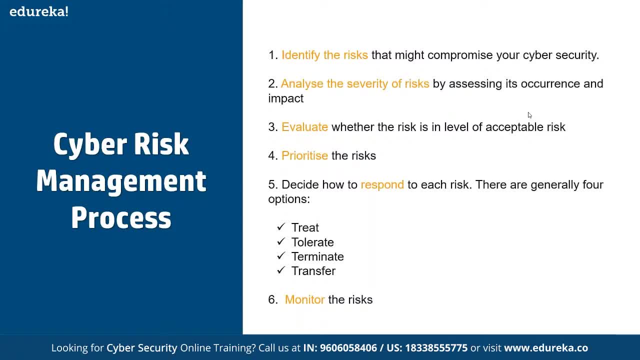 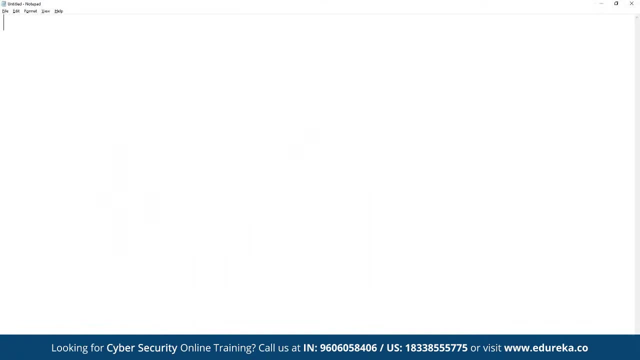 So we had discussed on the concepts of the recommendation by Deloitte as well. So if we talk about that particular process, so let's move to a notepad for having an understanding on that. So we had this kind of Deloitte recommends. 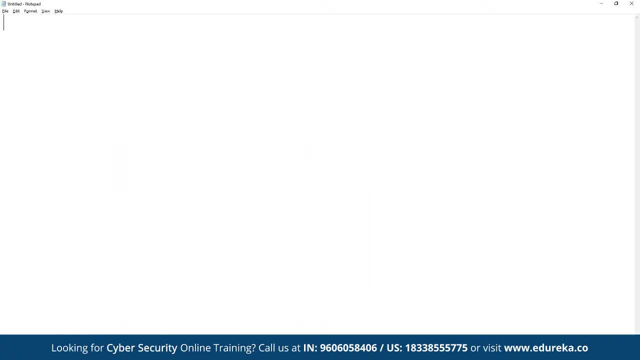 at risk management process follows the capability maturity model. So here we have something called as capability Maturity model approach. So basically in this model we have five different levels. So first of all we have the initial level, then we have repeatable, 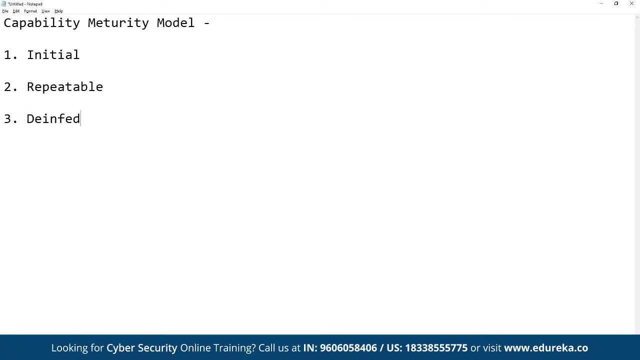 Then we have defined, Then we have managed and then we have the optimizing. So, basically, if you talk about the initial- or we can also call it as the chaotic, ad hoc or individual Heroic says- well, so this is going to be a starting point. 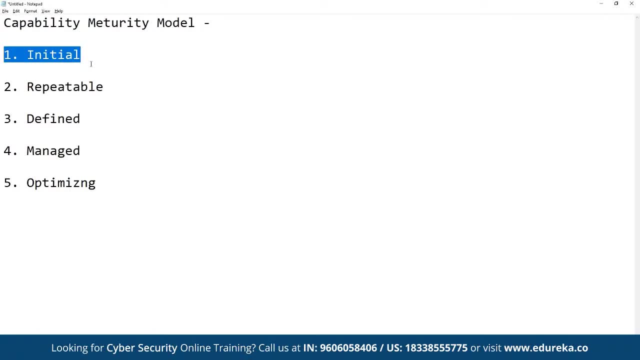 for use of a new hour: undocumented, repeated process and repeatable. if you talk about the repeatable part, then it is a simply a process which is at least documented. It's sufficiently such that repeating the same steps may be attempted. that, if you talk about Define. 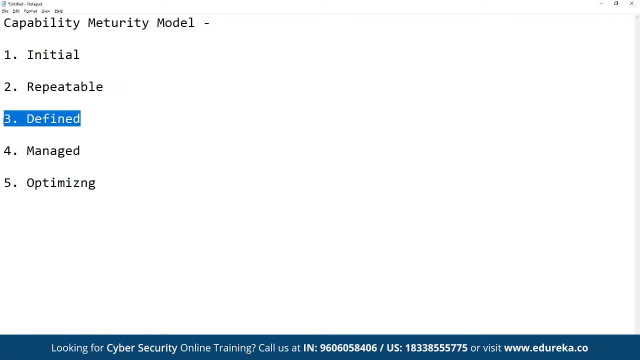 then Define is a process that is defined and confirmed as a standard business process. And then we have managed, which is basically the process is defined and the confirm. again, It is simply the process which is defined and it is going to be quantitatively managed. 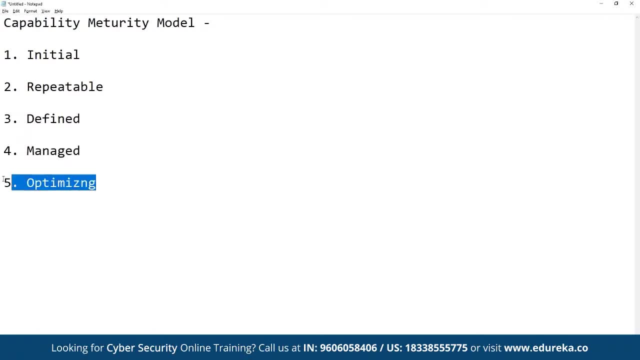 in accordance with the agreed matrices. And then we have optimizing, which is going to be the process management, where it is going to include deliberate process optimization or any kind of other improvements which may be required. So there are multiple other recommendations also made, like, for example, 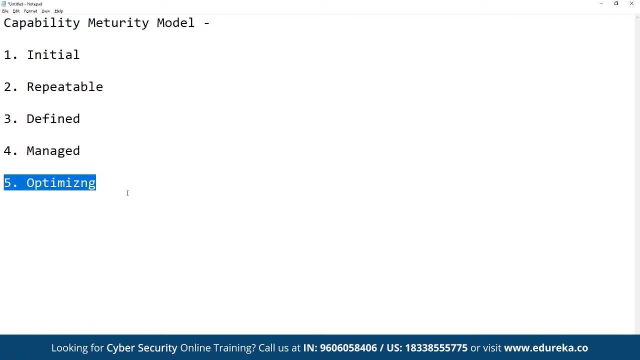 Deloitte also recommends using a risk-reward calculation and then prioritizing those Network security enhancements that will provide the greatest improvement at the lowest cost. now, some enterprises may be comfortable with 99% of all security upgrade being made. others, particularly in regulated Industries, will want to be closer to 100%. 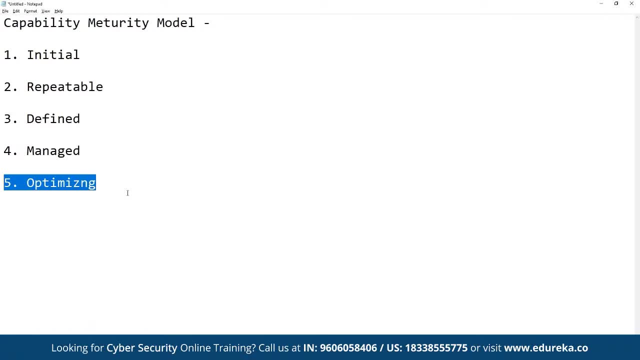 so there should be an incremental steps and goals. that is, 5% improvement within six months. that can be measured to determine if the enterprise is progressing towards its plan. cyber security risk washer. However, the even small security vulnerabilities can lead to large losses if Network systems are connected. 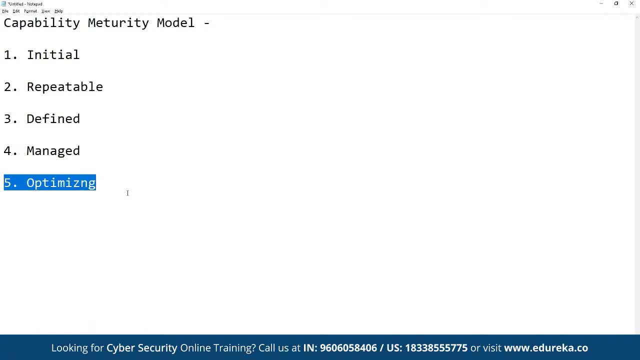 in such a way that the intrusion into an unimportant area can provide an unauthorized entry into more important systems and more sensitive data. So the only way to make a system 100% secure is to make sure that it isn't accessible by anyone, which is impractical at best. 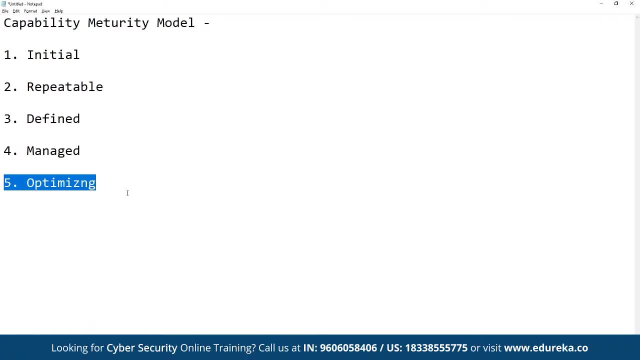 but we know, because if you want to make it 100% secure, then we can simply lock it down. But again, if the system is completely locked on- and obviously there is not- this is not going to be a practical way, because the system is meant to be used by the users, correct? 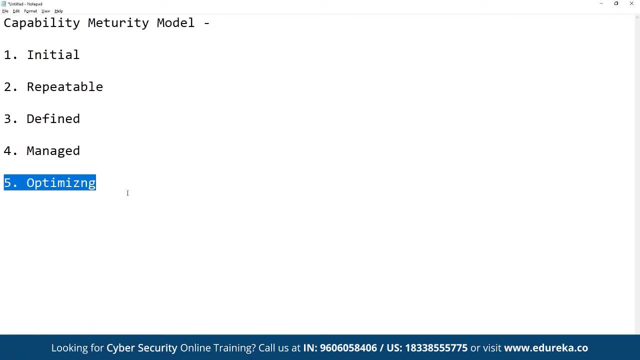 if they are not having the access, and then there is no purpose of building an application. So the more lockdown a system is, the harder it becomes for an authorized personnel to conduct the business. We know that right. So if authorized users find they cannot access the systems, 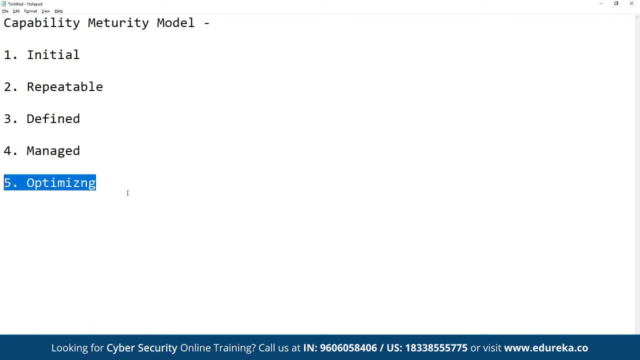 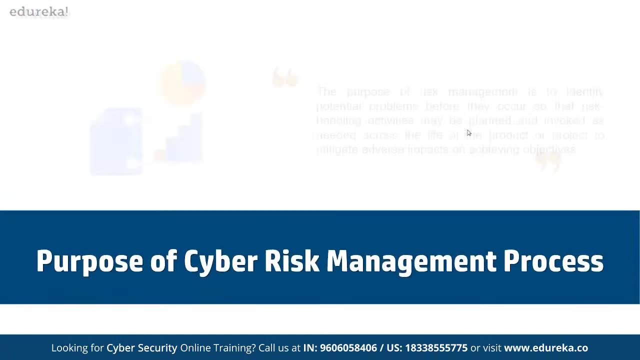 or data they need in order to perform their jobs. they may look for workarounds that could compromise systems. That's how it generally is structured. So now let's proceed further. The main purpose of the cyber risk management process, as we discussed, is: 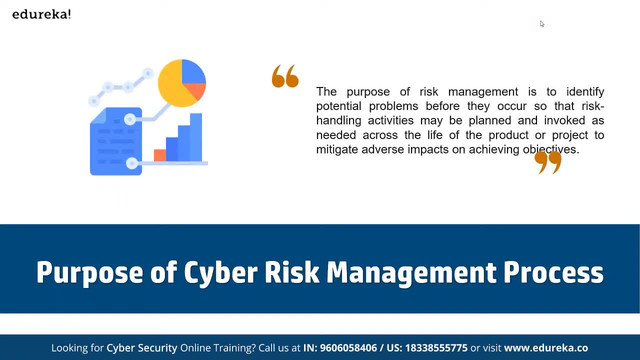 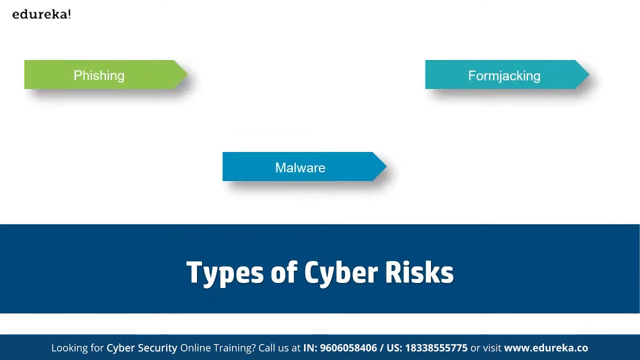 to identify potential problems before they occur, so that the risk handling activities may be planned and invoked as needed across the life of the product or project to mitigate adverse impacts on achieving objectives. So now, if you talk about the different types of cyber attack, so we have fishing, we have malware. 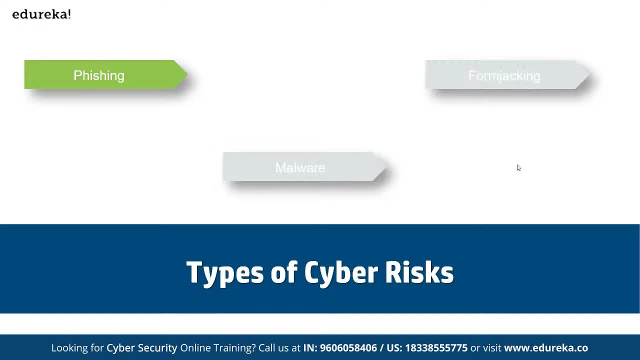 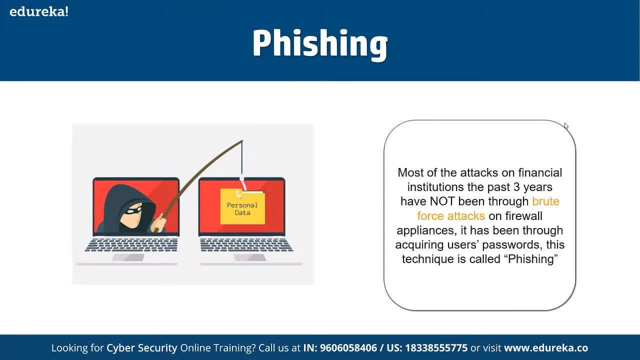 and then we have form jacking. So if you talk about fishing, then fishing is one of the most of now, most of the attacks on financial institutions. again, the past three years have not been through brute force Attacks on firewall appliances and has been through acquire users passwords. 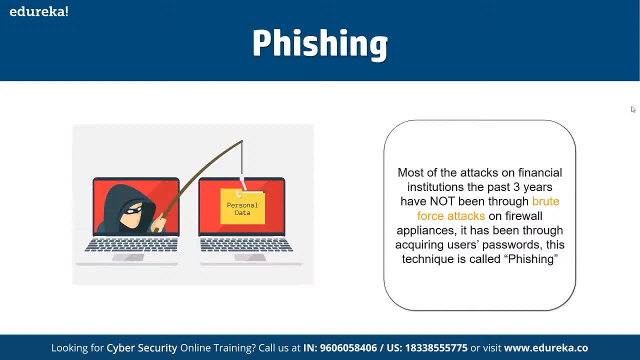 and this technique itself is called fishing. So simple example: let's say we have been. now we are going to log into any banking system. Let's say we are trying to log into a bank. Now, for example, we are trying to log into, let's say, SBI bank. 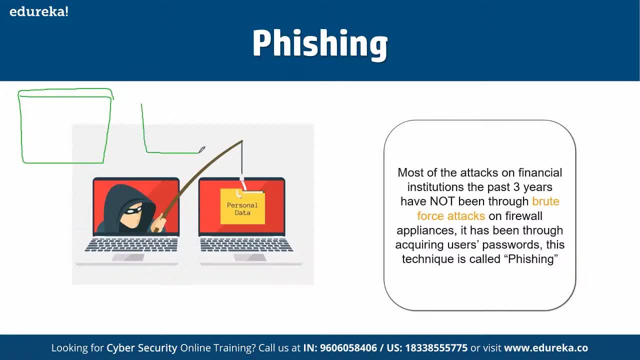 or, for example, it's a online SBI or we are trying to log into. suppose HDFC bank now features what they do? They simply create a similar looking page which is not going to be the actual page of the bank. Now the similar looking page is going to have the exact same. 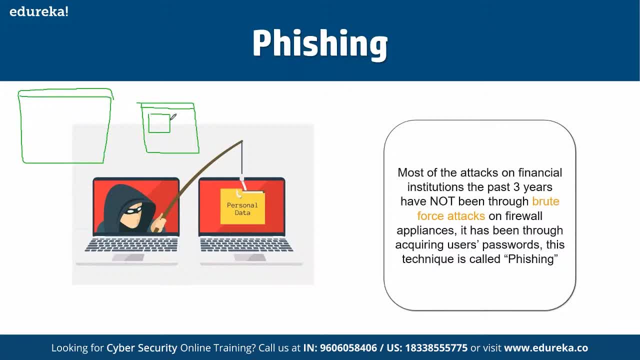 layout right. So they are going to have exact same layout with no differences, But again they'll be some, we can say, my new differences in the domain You are a little bit that we are going to see here and that is going to result in, and that is that free is going. 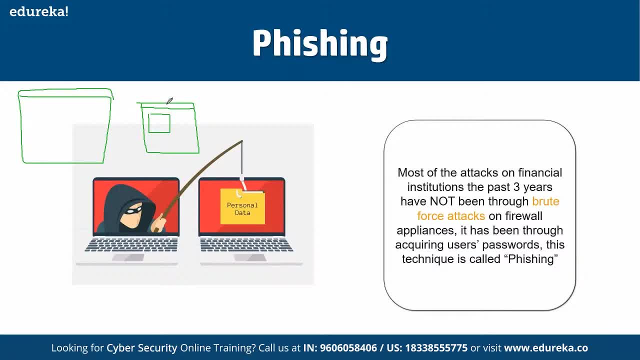 to result in users believing that the kid they are on the original page, and then they are going to enter their credentials and as soon as they enter the credentials they are that credential is going to be recorded by the hackers, and then that's how they are simply going. 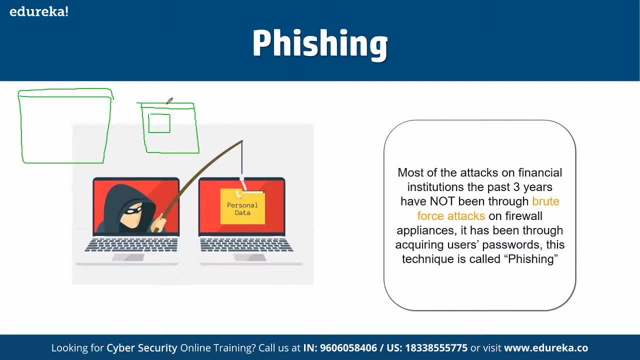 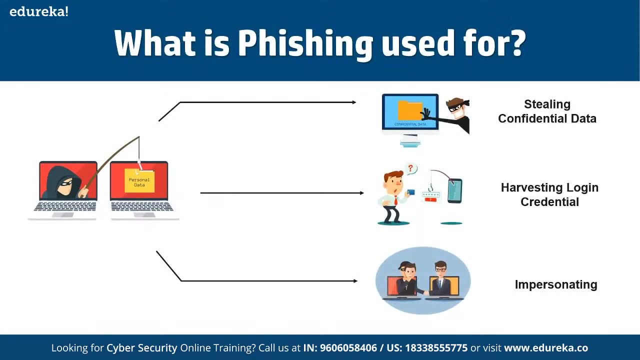 to get the password and the username for account, which we are going again, which is getting compromised, All right, and then, if you talk about, let's first of all erase this up Now. next we have fishing. As we discussed, fishing is used for stealing confidential data. 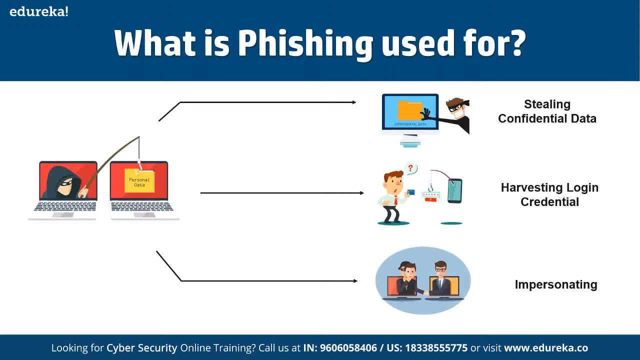 It is used for harvesting, logging credentials and for impersonating anyone, because I get out of the end. They simply in person, for example, a bank, they impersonate the bank King long because the login page and then they seal the login credentials and then, by using the login credential, 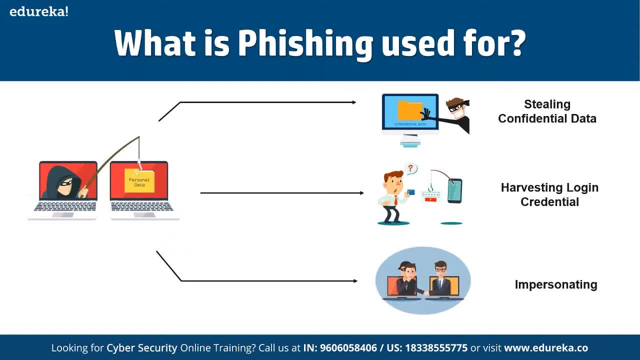 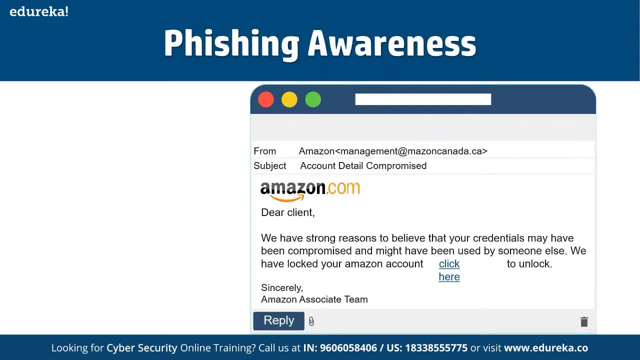 they seal the confidential data set or they can even make unauthorized actions And for example, a simple example- we can see how we have amazoncanadaca. Now this is an email received from amazoncanadaca, But again, if you pay attention, 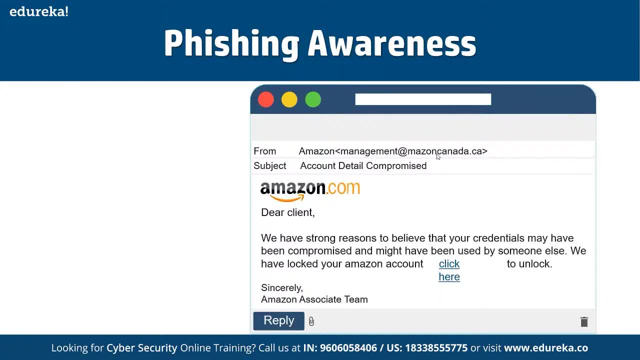 then this is not amazoncanadaca, It is mazoncanadaca. Now it's looks like the same because majority of the people they recognize Amazon. They don't focus much on the actual letters, right? and then they are currently using Amazon logo as well. 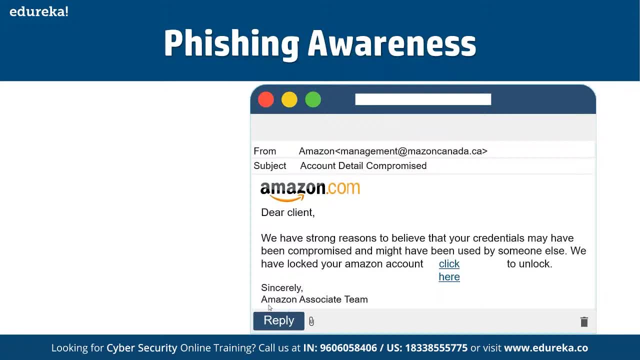 They are simply using the structure of the email followed by Amazon as well, And they are using a signature for Amazon associate team as well, And then they are simply asking that they should be, that they should simply reset the password, and the link that they have entered here is not the original link. 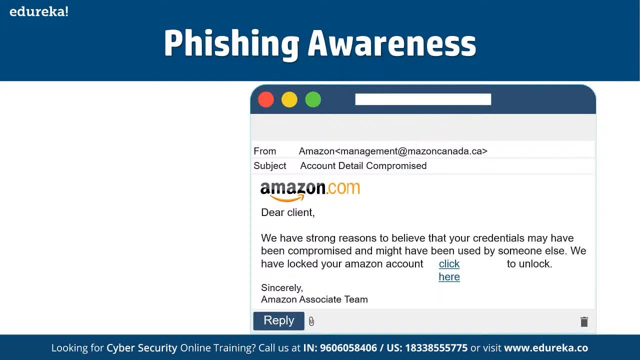 through which they can reset the password. This is a link which is going to take the users on the pay or the pages, or kids on the customized page designed by the attacker itself, And then they are going to enter their details And that's how this information is going to be stolen. 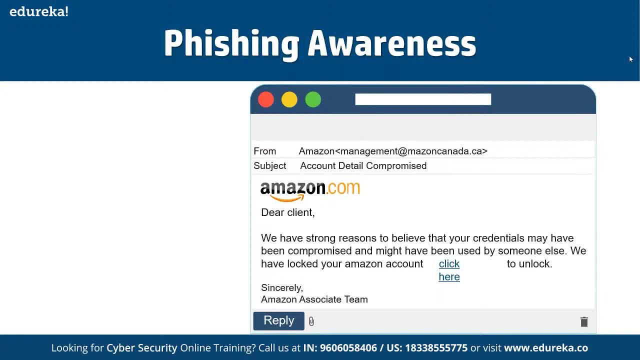 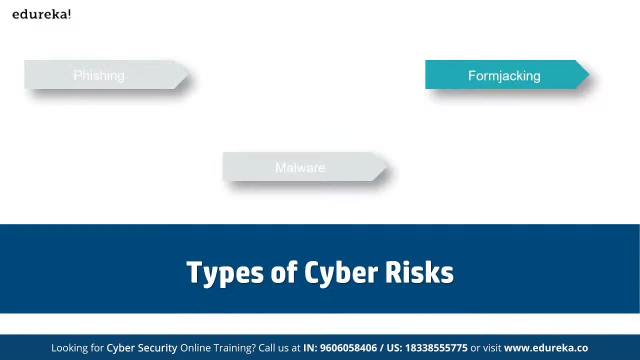 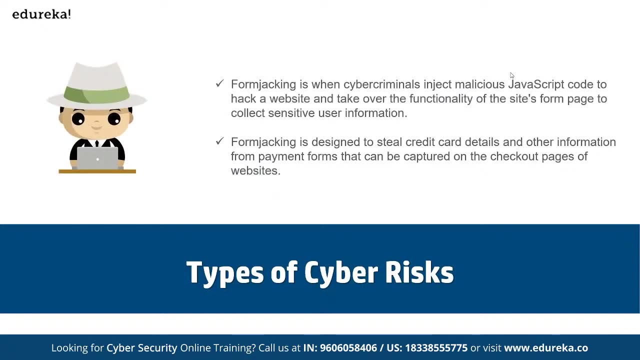 by the hackers itself, And that's a simple and plain example for fishing, All right. Next we have something called as form jacking. So if we talk about form jacking, then form jacking is when cyber criminals they inject malicious JavaScript code to hack a website and take over the functionality. 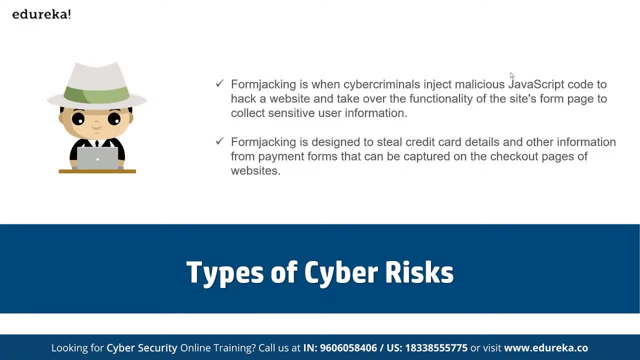 of the site's form page to collect sensitive user information. now, form jacking is designed to steal credit card details and other information from payment forms that can be captured on the checkout pages of the website. So that exactly is what form jacking is. So a simple example is: now you may not form tracking. 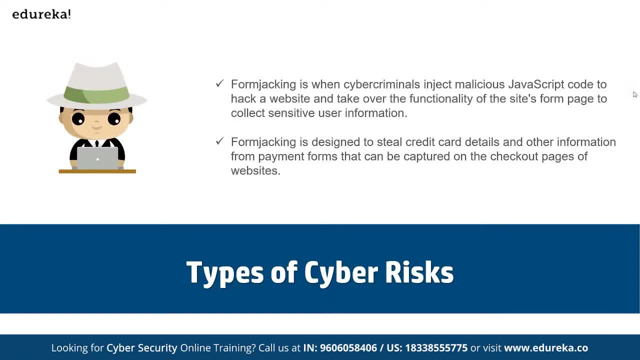 is also used in the comment section as well. So, for example, you may have seen multiple blogs, right? So blogs, They simply allow the user Just to add a comment on the session, on the on that particular post as well, and we may have a login detail as well, right? 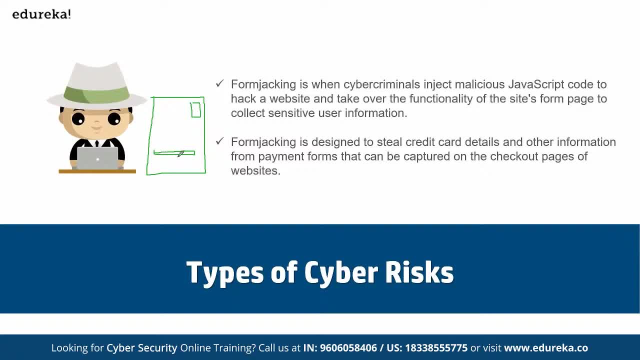 So form. so again, what hackers they do they simply if the JavaScript is allowed in the comment section. so they are simply going to inject their JavaScript code in the comment section and through this JavaScript code they can start getting details or this page as well. So, for example, they can get the entire website statuses. 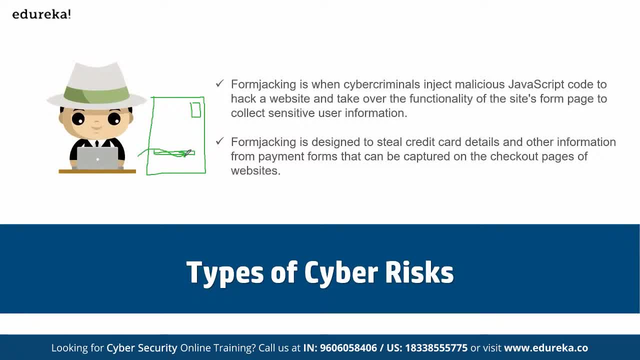 as well, just like we have in Google Analytics. Okay, What is the traffic? What is the number of page views? How did how exactly the traffic is coming into this page, along with allowing them to track the activities done by the users on this page? 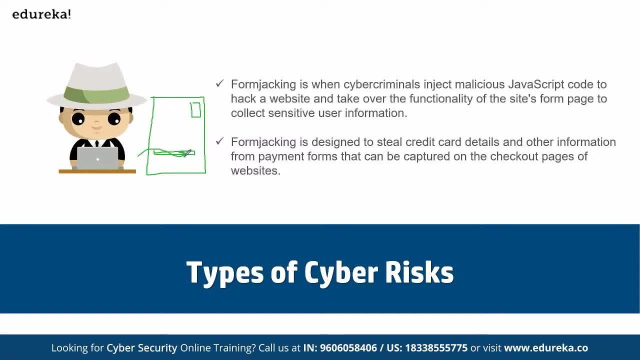 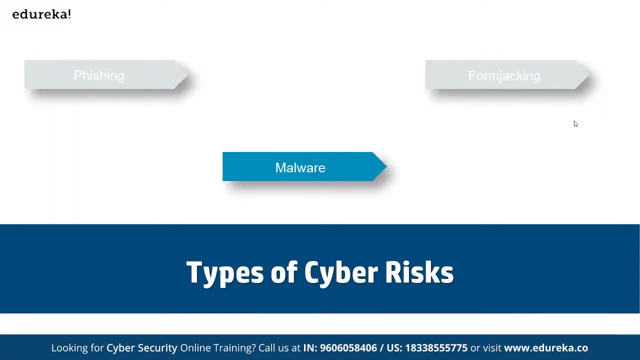 So that's why it's always a good practice to disable the inclusion of any kind of code in the comment section to avoid this kind of form-checking attacks. All right, So now let's proceed further. next we have malware, So malware has been one. 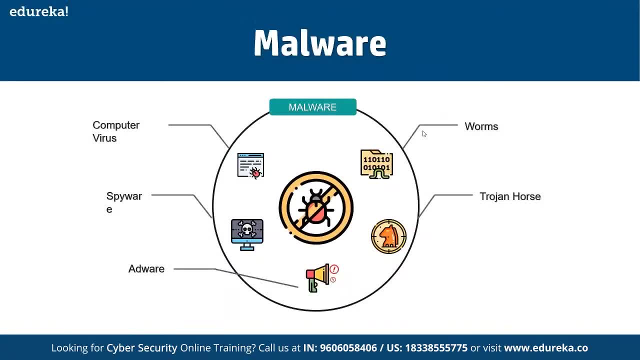 of the most popular attacks. So malware includes worms, Trojan hose, adverse spywares and the computer world virus. So the main job is to simply hack the system's data and they simply send the data enormously back to the users, and again, with and apart from just hacking. 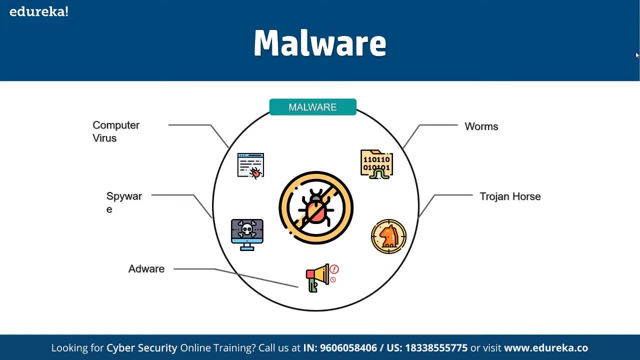 and keeping a track on the entire record set is simply, in fact, the system as well, with having certain kind of functionality disabled, or they simply trigger any kind of events, and that too, At a schedule Type, so that these events are going to occur again and again until unless we stop them manually. 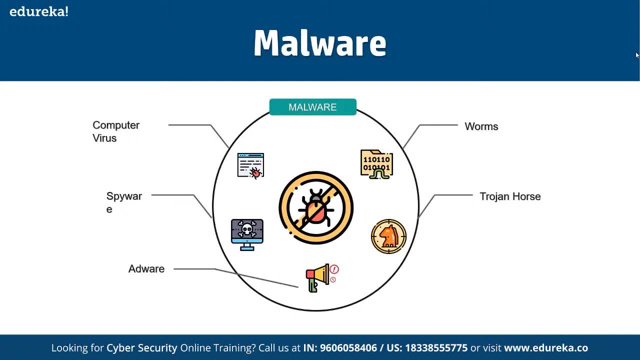 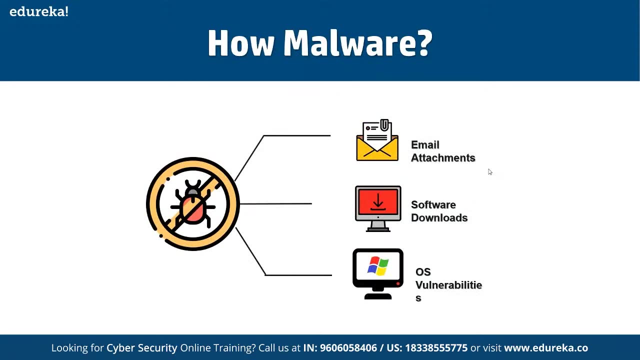 And these are the most popular task types that we have in Sabbath in the internet world right now. So how exactly the malware reaches- we can say reaches the systems. First of all, the most common way is through emails and that's how you may have seen the multiple emails. 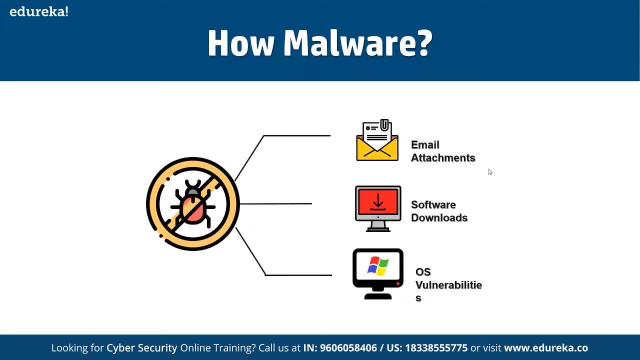 which contains multiple attachments, or they may be a blank email as well, in which multiple attachments can be added. and then it also arrives with software downloads as well. So majority of the of the cracks, the keychains that people download in order to bypass the licensing part again. 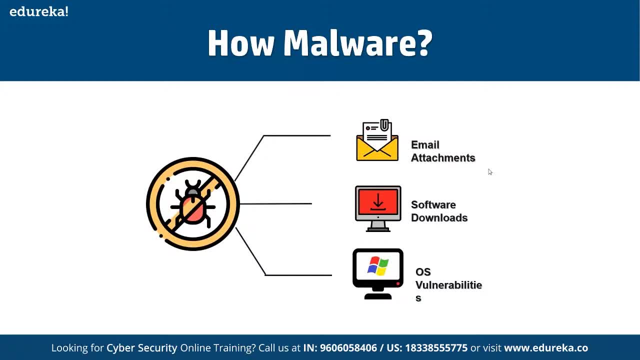 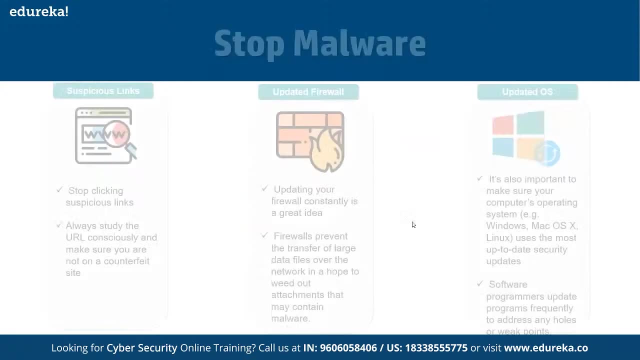 They already contain multiple viruses to help us in installation of those softwares, and then we have multiple OS vulnerabilities, So we can also get the virus through any kind of infected external hard disk or the USB drives or any kind of other connectivity Which may may have. and how to stop malware. 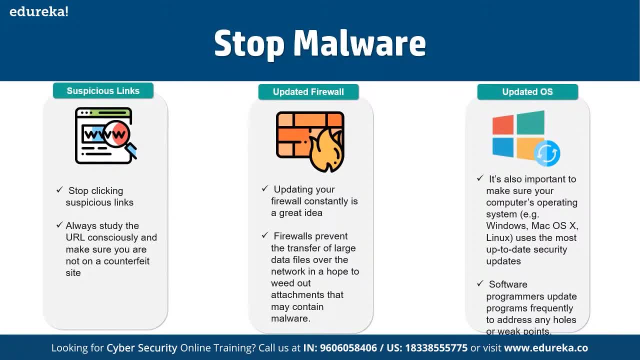 So we always have to ensure that we are stopped. We just simply stop clicking any kind of suspicious link, and we always have to study the URL consciously and make sure that we are not on a counterfeit website because, again, if we enter details that we have to simply bid adieu to our account. 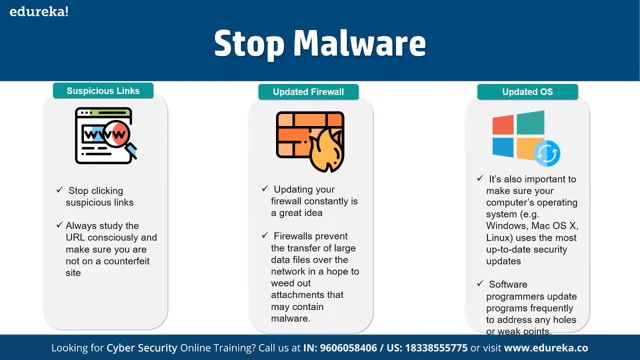 and then we have to always update our firewall because multiple new viruses They keep on, they keep coming on and on and that's why we have to ensure that our firewalls say as updated, so that even a new virus has been released into the market since the database has been updated. 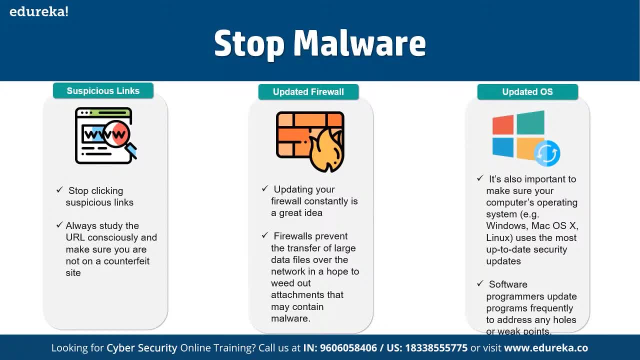 So that new virus is also going to be blacklisted in the firewall itself. So the firewalls are simply prevent the transfer of large data files over the network in a hope to weed out attachments that may contain the malware, and then, in terms of the OS security, 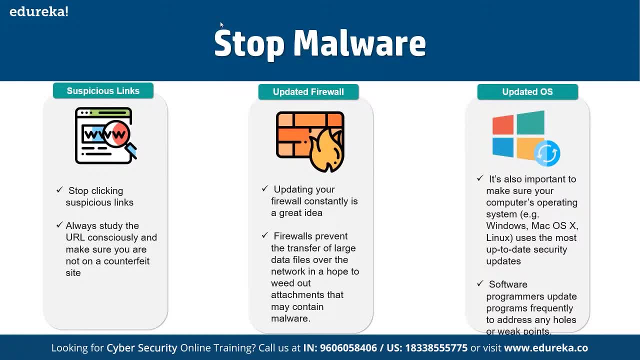 We always have to ensure that OS is continuously updated. So it's always so important to make sure that our computers operating system- example- We are running Windows, Mac OS or Linux- They all are using the latest version because the companies are simply keep on releasing multiple security patches. 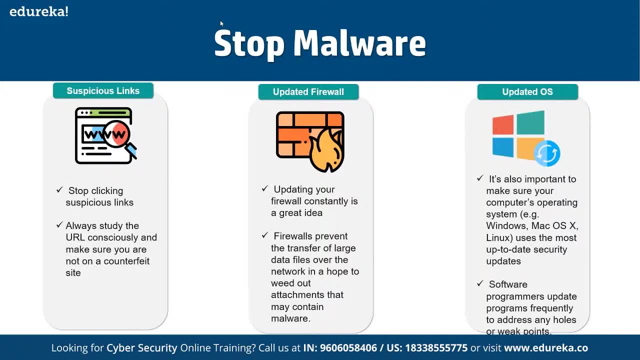 with the last updated virus, For example, there is a new security breach. They are new vulnerabilities record found on the OS, then again in the old, in the given OS. then they are simply fixed from those by, And those patches are required to be installed on regular basis. 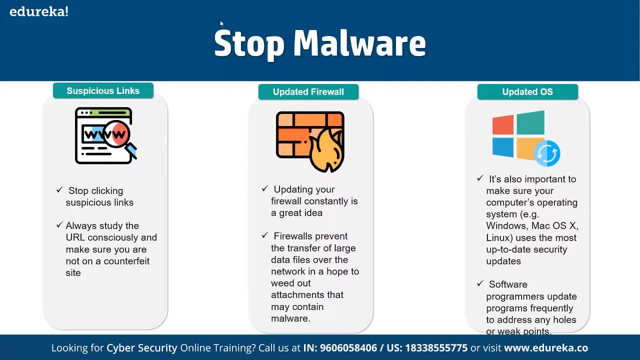 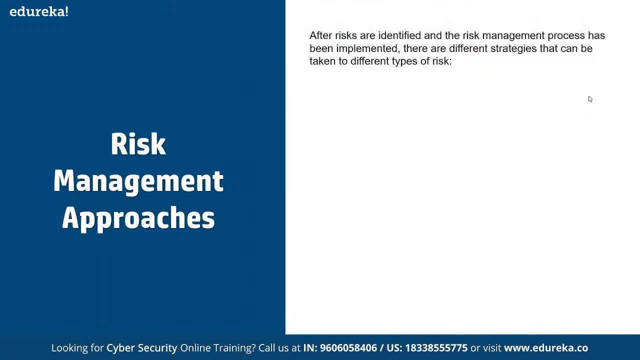 and software programmers. They update programs frequently to address any holes or weak points that may be exploited by the attackers. All right, So next we have risk management approaches. So after the risk are identified and the risk management process has been implemented. They are different strategies that can be taken to different types. 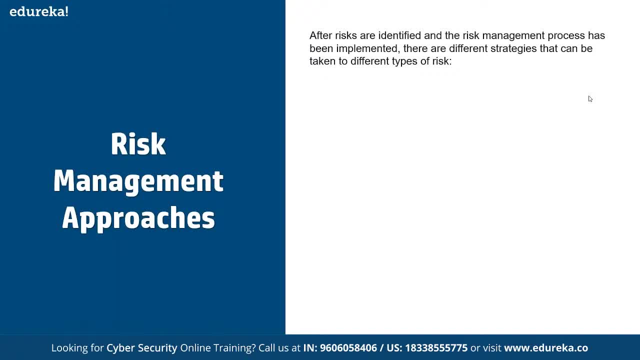 Of risk. So first of all, if you talk about the risk management, Then here we have to work on risk avoidance as well. So it's a famous proverb that to be safe than sorry strike. So here we have to ensure that we are keeping the entire updates ready. 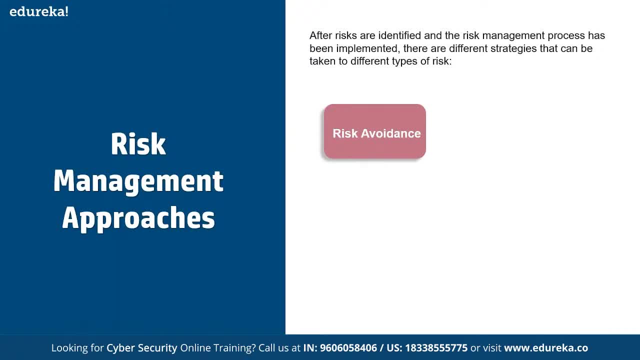 and we are simply making sure that they are no security breaches so that we can avoid having any kind of of attacks on system. And then here we have to reduce The risk reduction as well in making sure that, even if the attacks happen again, the possibility of a huge amount of data loss is reduced. 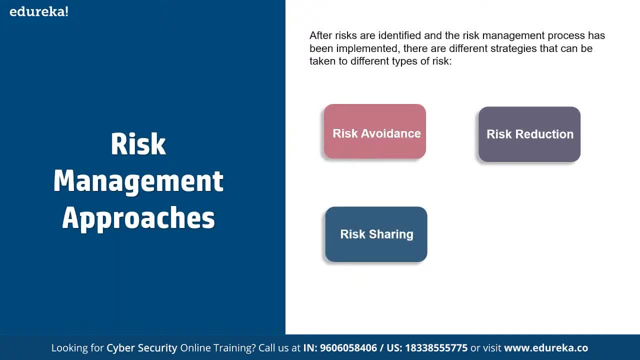 and then we have risk sharing. that means, instead of deploying the internet entire content and only one single infrastructure, We can simply share the entire application among multiple infrastructure so that if one facility is attached, still it can, still we can have in the application up and running will be having our data safe. 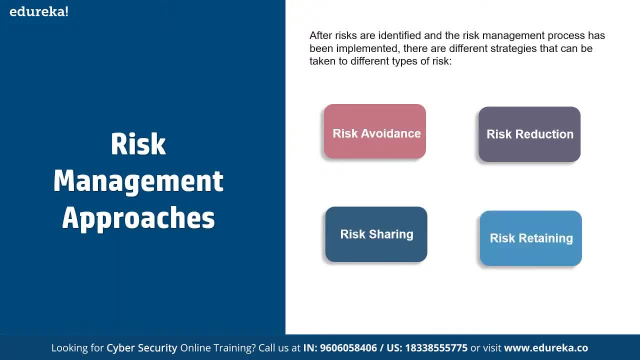 and sound stored in some other hardware As well. and then we have to retain the risk as well. as suppose, in case of any attacks, the damage should be minimum. So that is what we mean by risk retaining, and there are multiple measures that we can put into place. 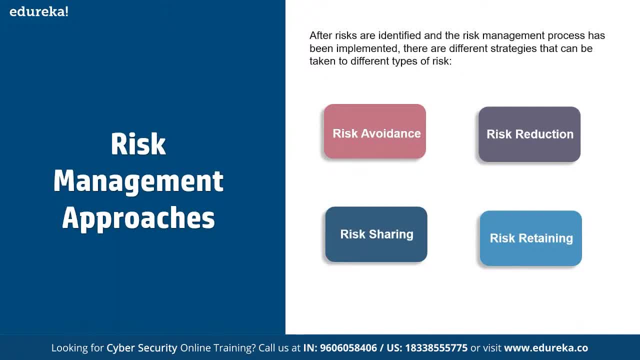 to avoid these kind of Situations and even if we are that and we are going to simply minimize the damage as well, Because if you know that external and internal attempts will be made to attempt to compromise an organization's data right, So we should always have the incident response plan. 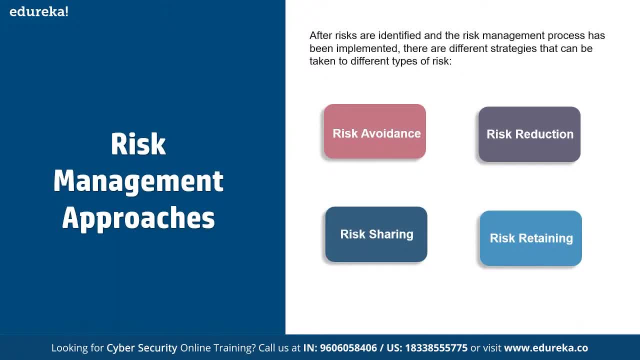 in place to determine what actions to take if the certain incidents occur. So an increase in a can hacker attempts at the enterprise or in the company's industry could mean the heightened precautions to be taken. So if an actual breach occurs, the enterprise should have detailed plans. 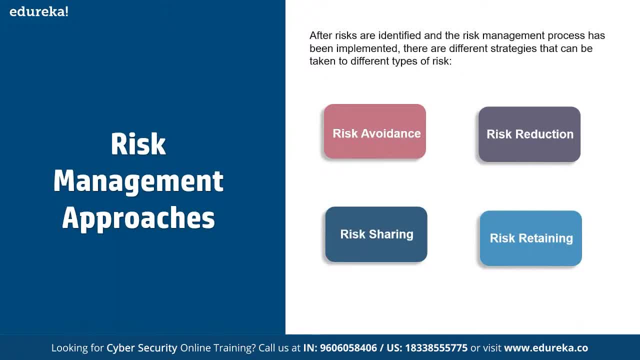 in place for those for who to notify inside and outside the company, content Information for law enforcement businesses, supplies and customers. and action item checklist public relations sponsors- a truck and their multiple guidelines as available as well. That means what should be done in order to avoid these kind. 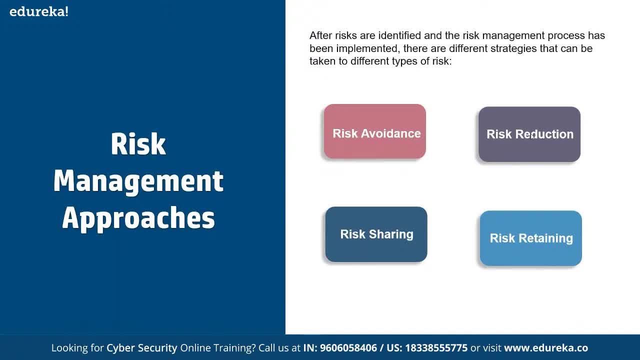 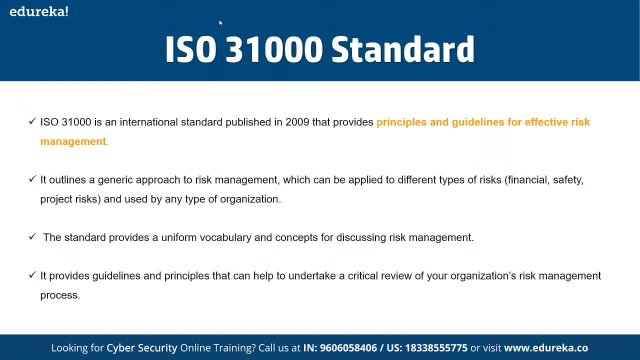 of attacks Now. next, we have the ISO 31,000 standard. So ISO 31,000 is an international standard, published in 2009, that provides principles and guidelines for effective risk management. So it outlines a generic approach to risk management which can be applied to different types of risk. 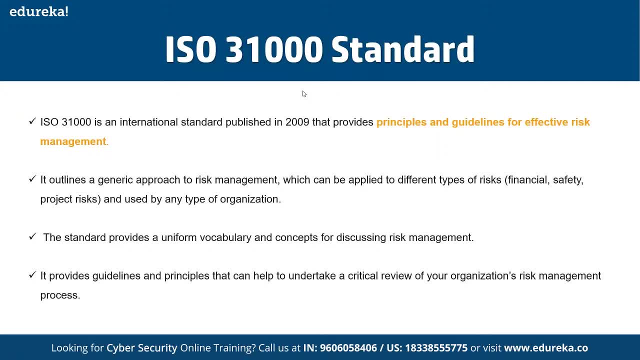 which can be financial, safety or any kind of project risk used by any type of organization. So the standard provides a reform vocabulary and concepts for discussing risk management. It provides guidelines and principles that can help to undertake a critical review of organizations risk management process. 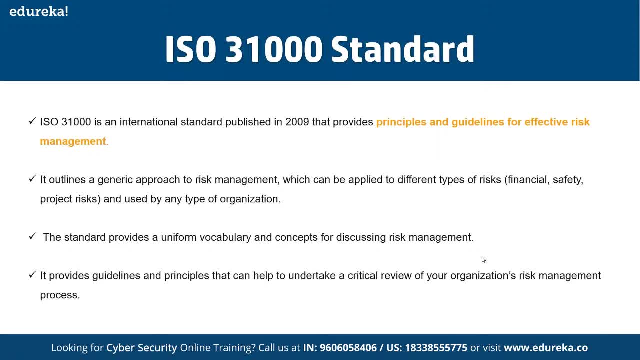 All right. so now there are multiple methods of risk mitigation as well. So among the cyber security precautions that we can consider, we can consider working on limiting the devices with the internet access. We can install the network access controls as well for securing the entire network all together. 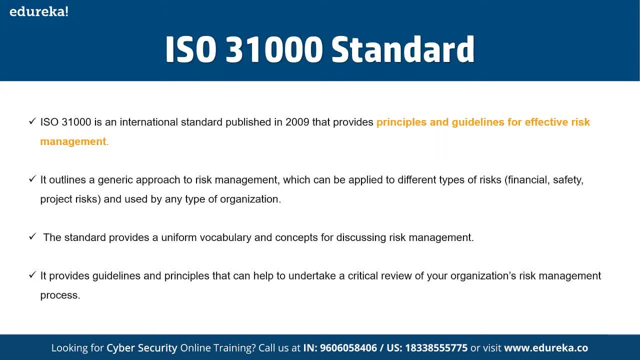 So if you talk about the network control access, that again here we have multiple process. if I under any see, we refer to it as NAC itself. So under network control access we help. we are simply going to implement multiple policies for controlling devices and user access. 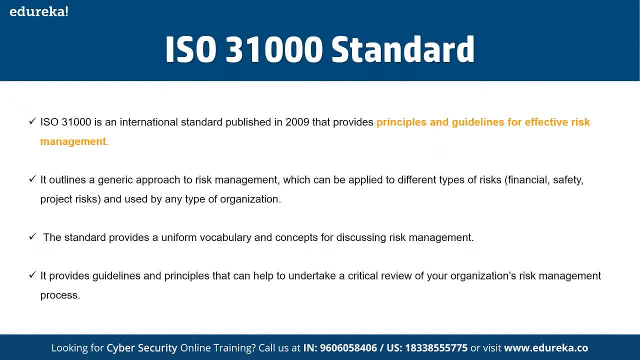 To the networks. so NAC, or we can say now, can set policies for resource, role and devices, as well as and when required. So NAC is basically offered to create outer or the chaos for the given Corrections from within and outside the company. For example, let's say, if we have been using multiple 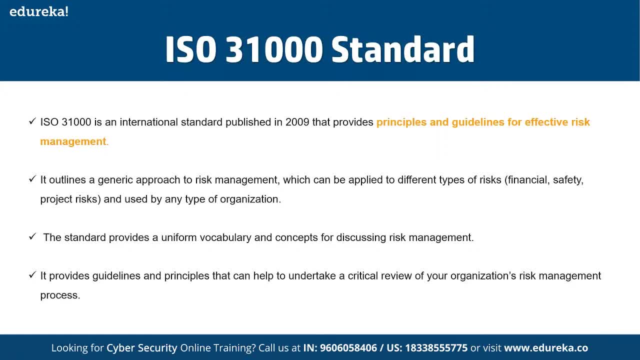 for cloud platforms. now, within cloud, we have services being offered. For example, we have services that we can make use of. let's say, we have a requirement of creating a multi-tier architecture. So obviously, when we are creating a multi-tier architecture, then we do have to ensure that we are creating a, we can say, a public subnets. 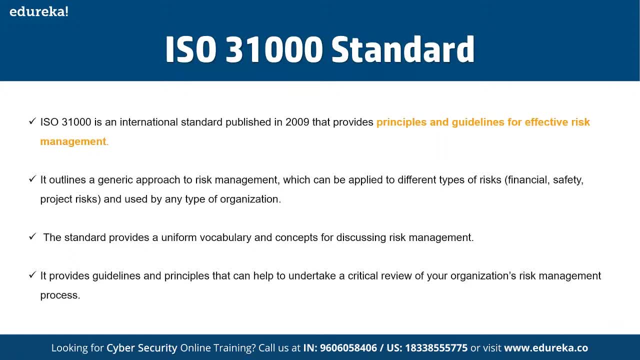 and private subnets so we can define the public subnets for the web servers where we are going to host the web server and where we would need to- where we do- To have the access to a public IP defined for every server that we are going to host here. 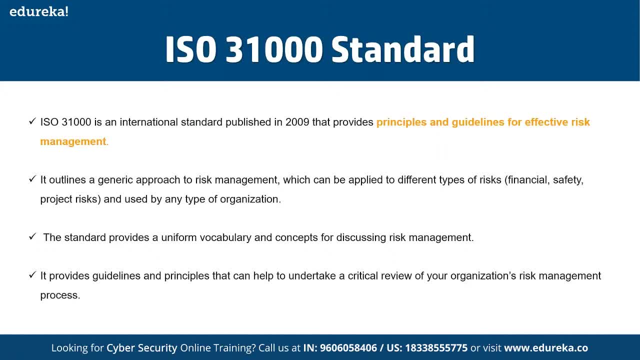 That's how to structured correct. same way, if you talk about the application servers, now, application servers, they are critical, right? they are critical components of the application. that means they are. they don't need to have any kind of public access defined, and that's why we have to ensure 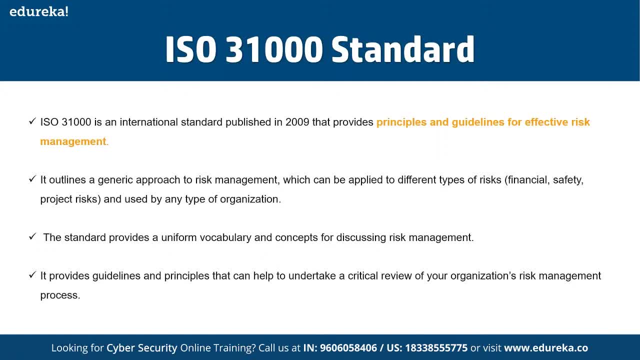 that we simply disable the public access, correct, and then we also have a again and same way. if you want, we can to find the database servers in the same private subnet as well, through which we can simply disable the access to the internet so that we can use the NAT gateway. 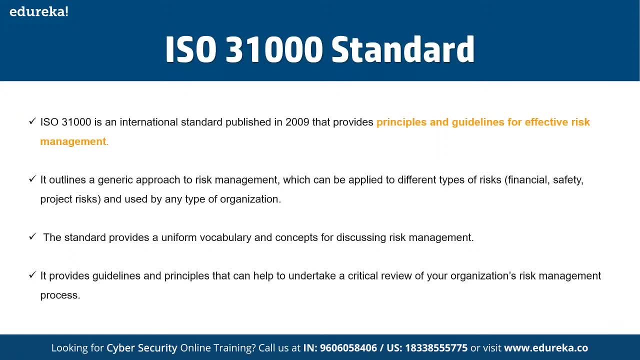 in order to work on multiple security patches and updates, then that can be done by using that gateways in order to have a complete control on the network. So there are multiple knack related process that we can go for. so same way here We have other risk mitigation strategies also available. 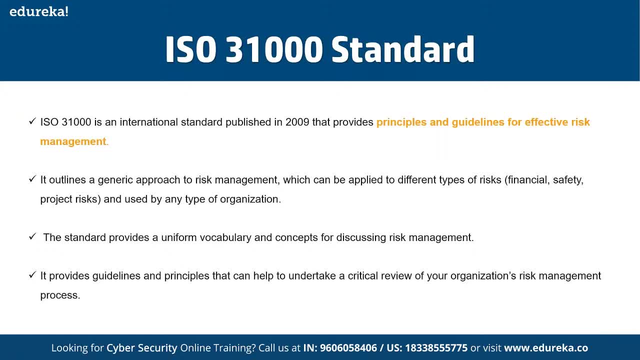 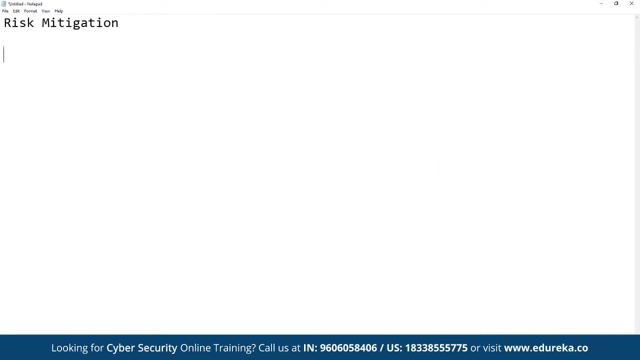 that we can go for. let me just list down all the mitigation techniques as well, so they can use it as a reference. We can also go for automated patches. Let me just list it down. All right, so in terms of the risk mitigation we can define. 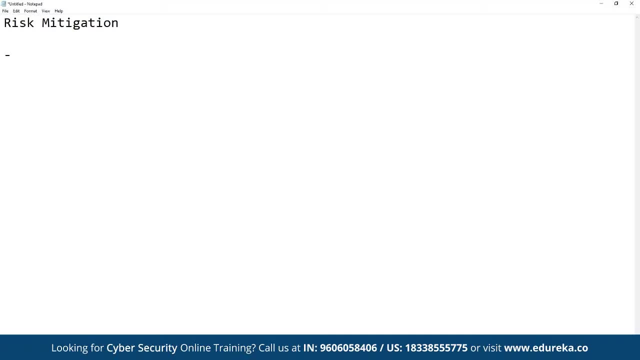 around here. We have you here. We had discussed first of all, we can focus on using the knack for having the network Access control. we can use that, then we can. We can make use of automated patches- automated Patches for the operating system. 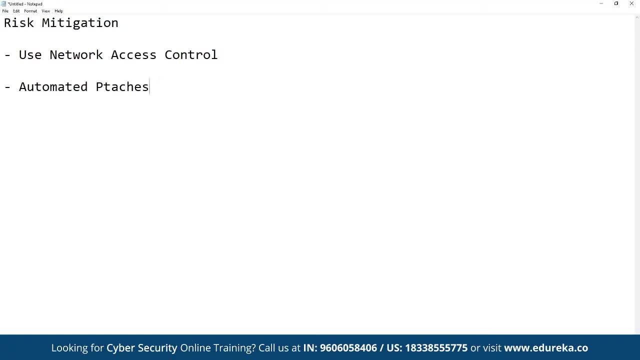 So basically, we get, define the product, whatever patches, whatever security patches needs to be there. So they're getting. we have to make sure that we are having a regular update done because in case they have been some new vulnerabilities found in the operating system, then the patch is going to simply fix them right. 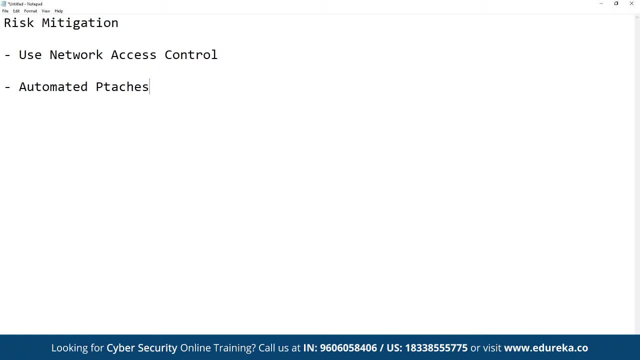 and that is what an important factor in risk mitigation is, because we are discussed at risk that OS are also highly vulnerable components in any security infrastructure, and then we have to limits when we have. we have to apply the limits for the older operating system as well. 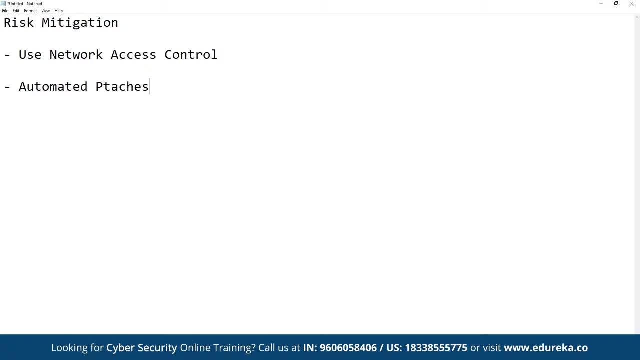 That means I get devices running Windows, Excel or older OS is not going to be supported. and then we have to ensure that proper firewalls are put into place, having a complete knack baseless and a security groups refined so that we can limit the access to only sudden IP addresses. 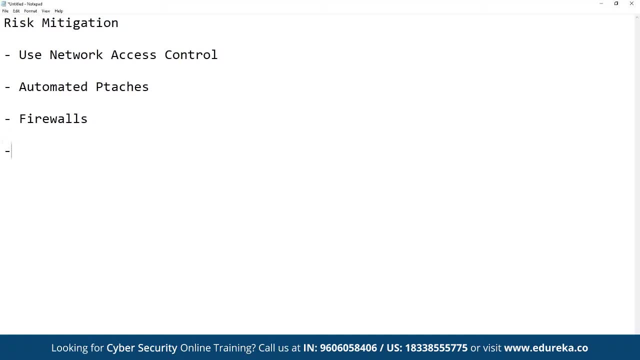 And then we should be having the two-factor authentication. So we have we can use two-factor or we can say MFA, as in multi-factor authentication. We have multi-factor authentication method defined. So using multi-factor authentication we can ensure that we are securing the user, the admin. 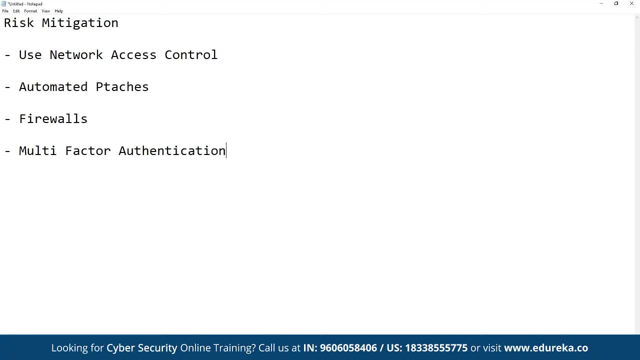 and the root user account, so that if anyone wants to get the access to these critical accounts, they need to have the access to a security code or device as a part of multi-factor Authentication process. right, and we can also make use of the advanced encryption. 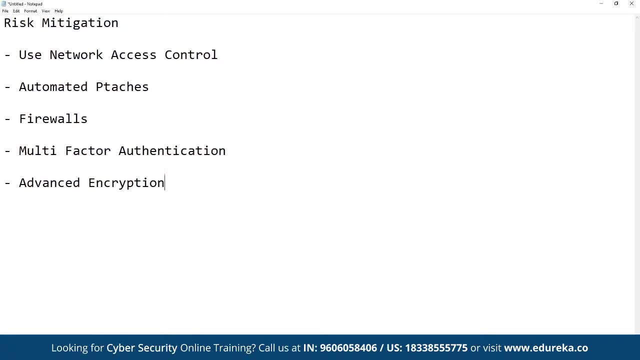 that we can implement now in terms of advanced encryption. So now, this is not a new feature in for, let's say, for databases, but today encryption must be implemented in a more strategic and systematic way to protect data from cyber criminals and other threats available. 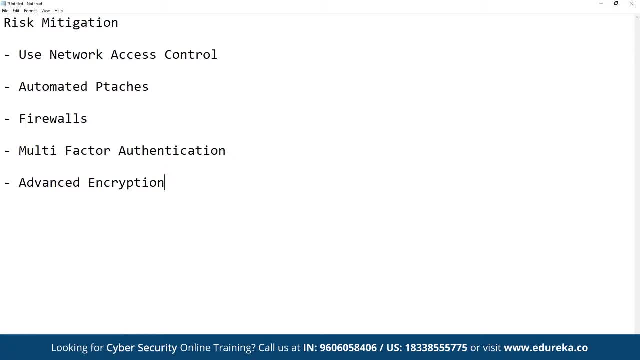 So this includes role-based access, standard-based cryptography, advanced key management. We can also go for the state-of-the-art algorithms. that is going to simply increase- or you can say increase- the security and decrease- the exposure for these components and through data encryption, We can have a control on the security breaches from outside. 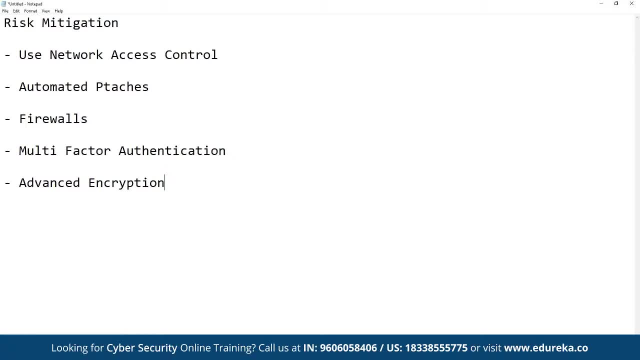 but it simply does little to prevent the internal Thrift. that's a drawback for encryption. So insiders, that means anyone having the account itself. So they are going to have the access to sensitive data Because you'll be having the credentials to decrypt it, right. 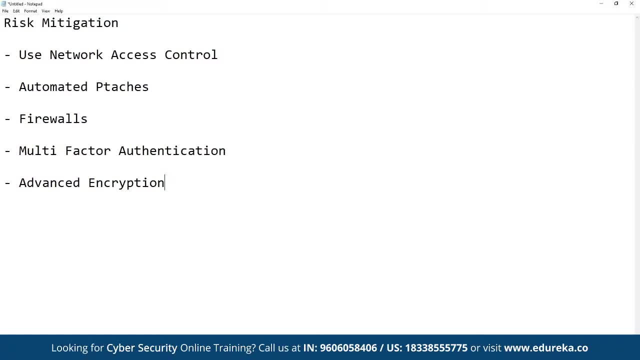 so companies that are working in a company. We also have to protect against data being removed from Enterprise systems through removable media such as thumb drives and other means. that's why these things are implemented right, And then we can also go for element level security as well.